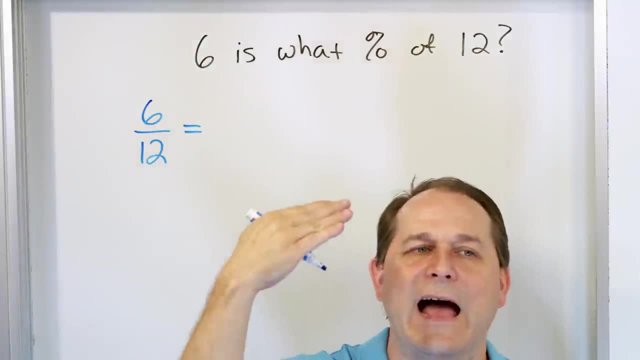 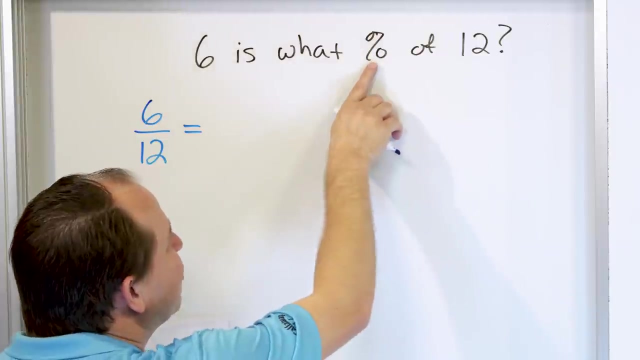 What does it mean to be a percentage? A percentage is how much of something compared to 100, right, Because that's what percent means. 50% is 50 out of 100, or 50 over 100.. 10% is 10 over 100.. 5% is 5 over 100.. Here we're trying to figure out what is the percent. 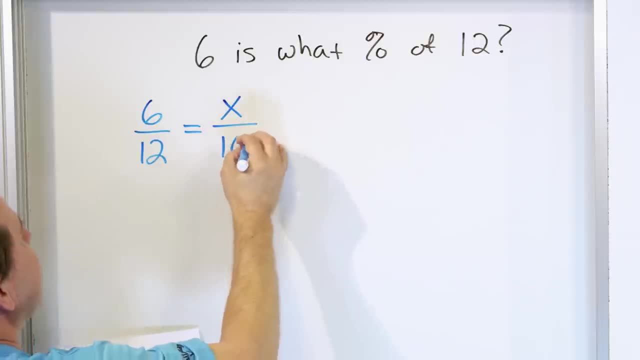 So we're going to call it x, an unknown over 100.. This is what we have to solve. Doesn't this look like a proportion? We already learned how to solve proportions before. I taught you over several lessons- four lessons actually- how to solve these proportions. So let's go ahead and start. 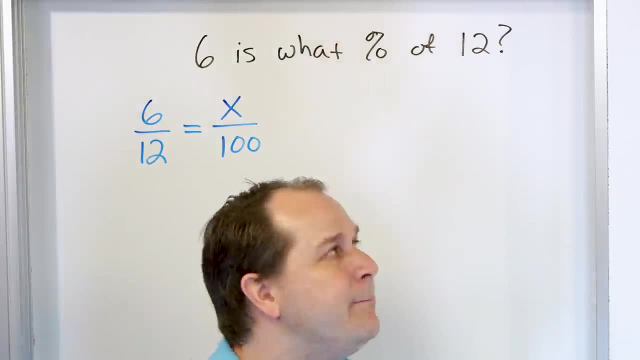 these kinds of problems. And now you're learning one reason why we did that: because we now know how to solve these things and they allow us to solve percent problems. So what we're saying is six, as it relates and compares to 12 as a ratio, is exactly equal as a ratio to some number out of. 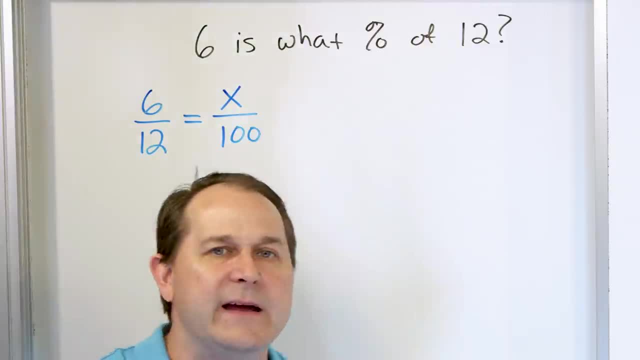 100. And when I figure out what x is, then it's out of 100. That means it has to be the same as the percentage, because a percentage is always out of 100.. All right, So let's rewrite what we have. 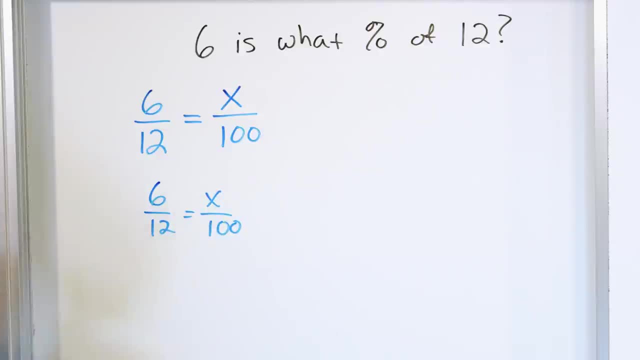 here. So we have 12 is x out of 100. All right, What do we do? Well, we want to get x by itself. Now we could just multiply by both sides by 100. That would kill the 100 that's here on the bottom. 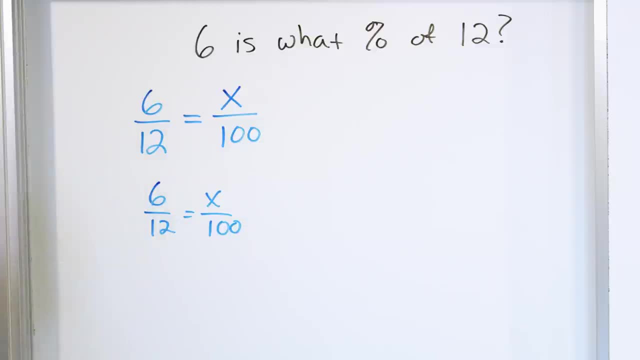 because it would cancel there. But let's think a little further. 6 out of 12.. We can already simplify this fraction. You see, any numbers that you can simplify or any fractions you can simplify ahead of time is going to make all of the calculations easier, So I always want you to try. 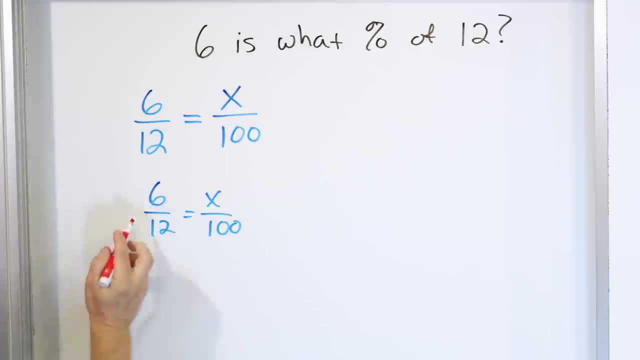 to do that. I can do that by simplifying the fraction. I can do that by simplifying the fraction. I can divide the top and bottom both by 6.. And I'll do that. I'll strike through and say 6 divided by 6 is 1, and 12 divided by 6 is 2.. So what I really have is kind of like a new related. 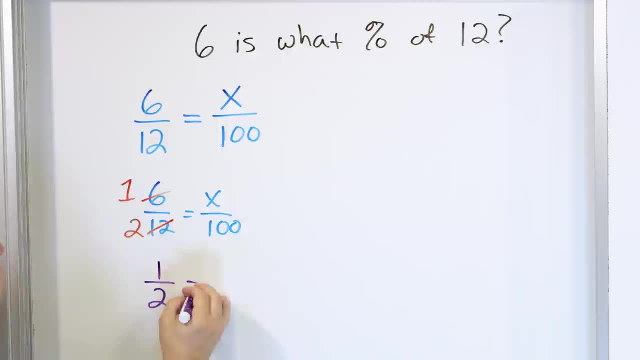 problem where the new numbers are 1 out of 2 is x out of 100.. This is exactly the same as this, because 6 12ths is exactly the same thing as 1 half. It's just a different. it's the same ratio. 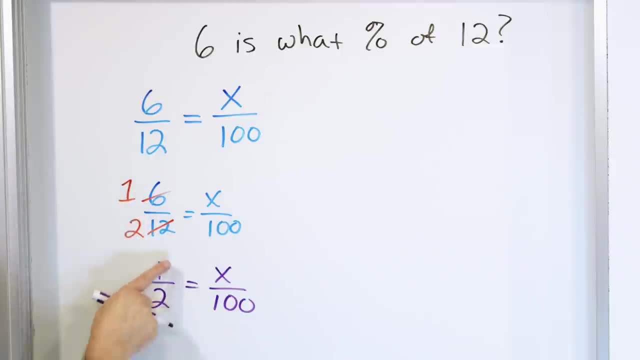 in other words, 6 12ths is the same ratio as 1 half. So replacing it with 1 half doesn't change anything. I'm just saying these ratios are the same. So next we can solve by doing what We're going to multiply by 100.. And if we do it to that side, 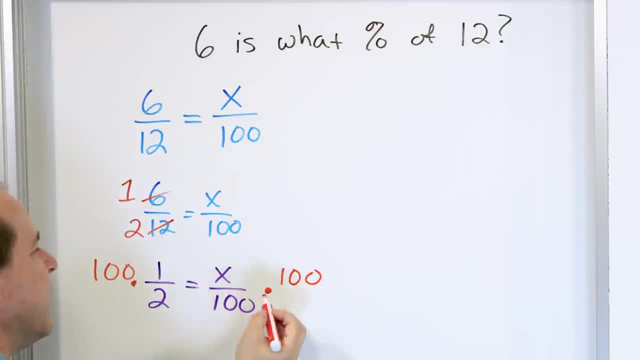 we have to multiply this side by 100.. Why are we doing that? Because now that we have 100 on the top, because, don't forget, this is like 100 over 1 here and this is 100 over 1 here, 100 on the. 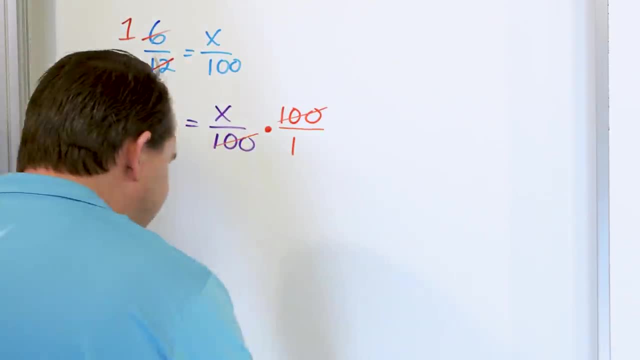 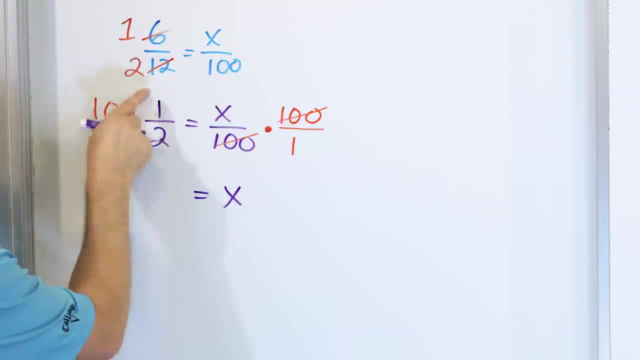 top and 100 on the bottom. I can strike through, And so the only thing that's going to be left on the right-hand side is just x. We're trying to get x by itself. On the left, you'll have 100 times 1,, which is 100.. And then you'll have 2 times 1, which is 2.. 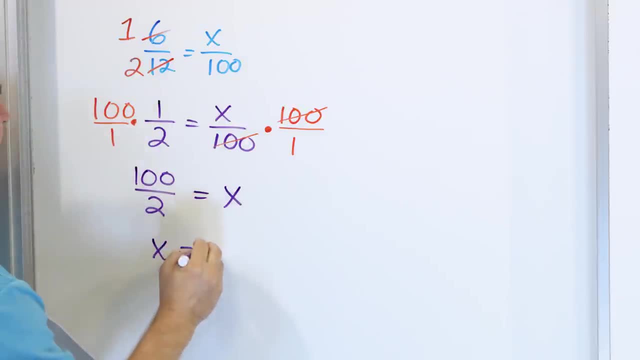 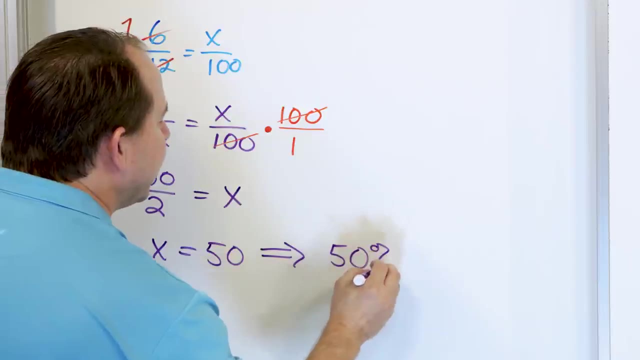 And then x, flipping it all around, would be 100 divided by 2, which would be 50.. x would be 50. So that means that 50% is the answer. That's what I want you to. circle x is equal to 50. Yeah. 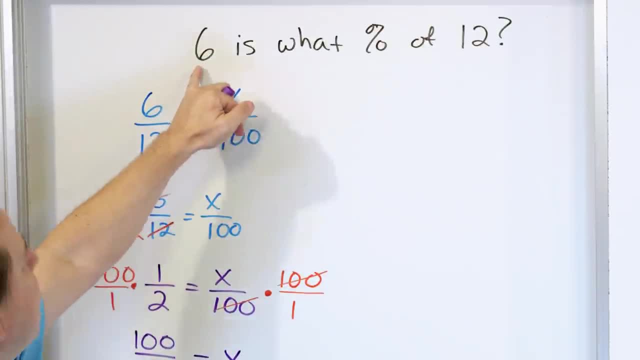 that's what we calculated. But don't forget, what we're trying to figure out is what is the percentage, And what we figured out is that, since x is 50,, 50 is what goes in this spot, 50 is the percentage that works, And so we're saying the ratio 6 twelfths is the same ratio as something. 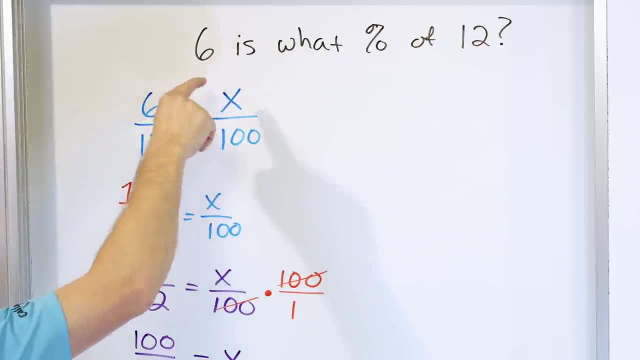 out of 100. And this unknown number came out to be 50. And since it's 50 out of 100, that means it's 50%. So that's what we're going to do: for every problem, We're going to set up a proportion. 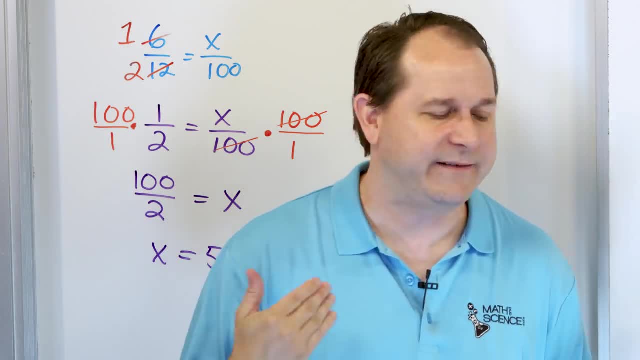 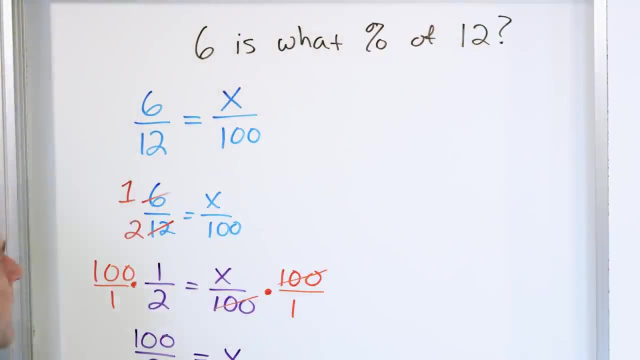 We're going to solve it, And then the answer we get will be the percentage. That is exactly what we're going to do for every one of these problems, And it makes sense, because we know that 6 has to be 50% of 12, because it's half of 12.. That's how we know that. All right, next problem: 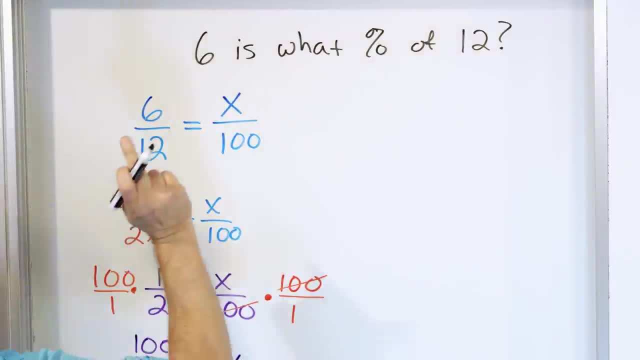 And also, I'll just point out one more thing here. When we were at this point, we could have just multiplied by 100 here and gone through all of the math, and we would still get the same answer. But by pre-simplifying this fraction the numbers were much easier to work with. That's the only. 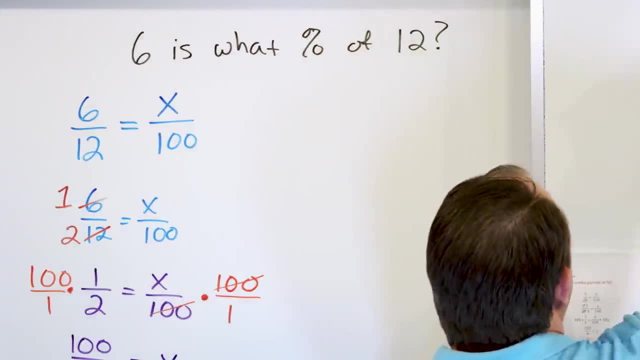 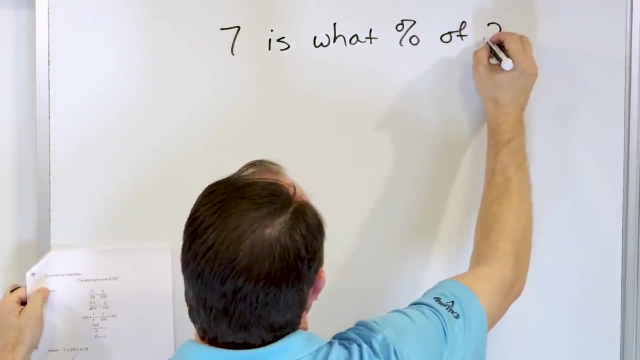 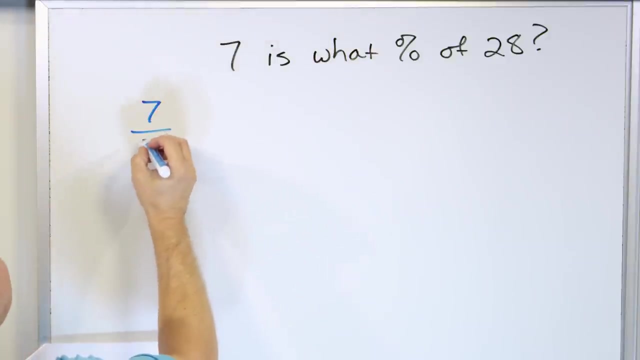 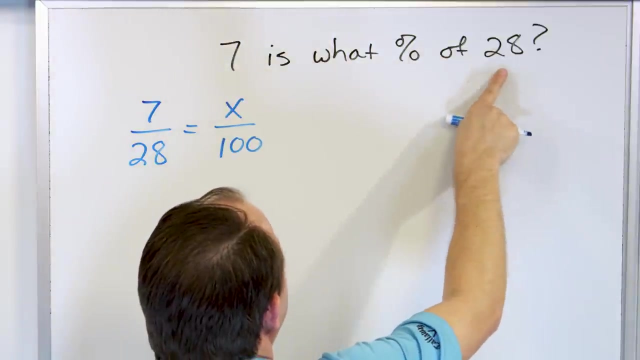 reason that you like to do that step. So let's take a look. 7 is what percent of 28?? All right, 7 is what percent of 28?? What we're saying is the ratio, 7 as it compares to 28,, is equal to some unknown number out of 100. Because 7 is what percent of? 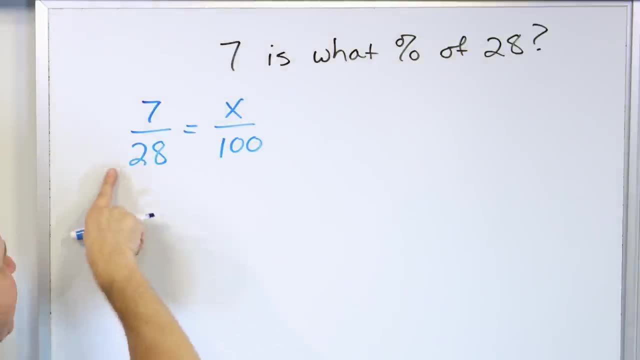 28,. it means 7 as it compares to 28, as a ratio, is equal to some unknown number out of 100.. And whatever this unknown number is will be the percentage. So let's rewrite what we have: 7,, 28, x 100.. Now we see a 7 and a 28.. We don't have to pre-simplify, We could just multiply by. 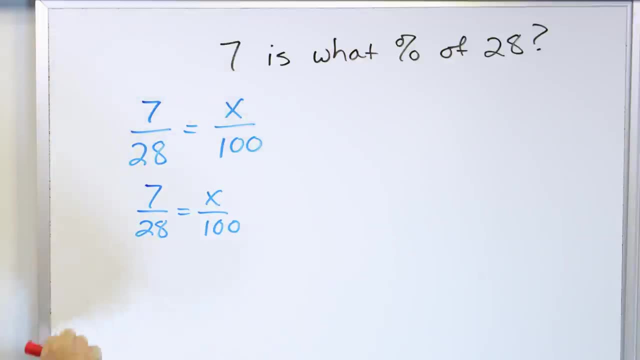 100 to get rid of the 100 and solve, But we'll have large numbers to deal with. So instead let's recognize: I can divide top and bottom by 7.. 7 divided by 7 is 1.. 28 divided by 7. 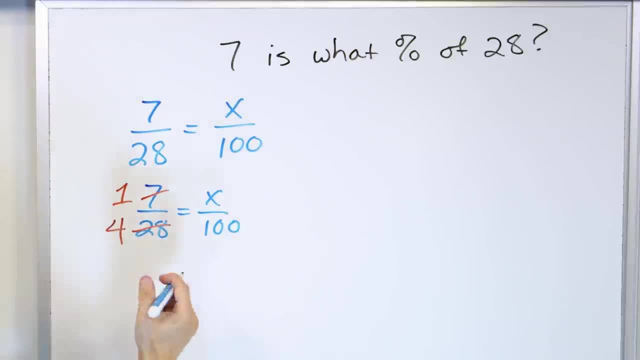 is 4.. And now I have a new kind of related problem, which is: 1 over 4 is equal to x over 100, like this. And now that we have already done this pre-simplification, this proportion is much, much easier to solve. So to get x by itself, we're dividing by 100.. 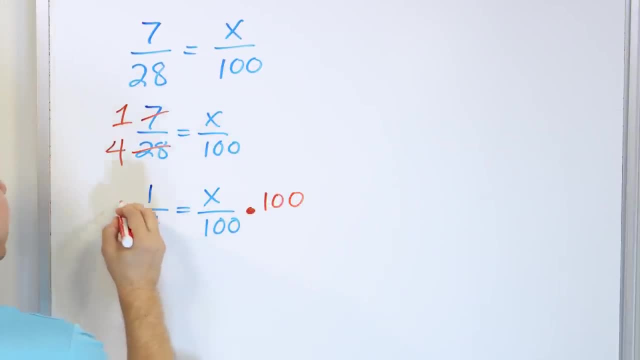 We'll do the opposite, which is multiplying by 100.. In fact, we're going to be doing this for every problem, basically multiplying by 100.. And you can see that, Don't forget, it's 100 over 1, and it's 100 over 1.. I think we don't have to write the over 1 every single time. You can see. 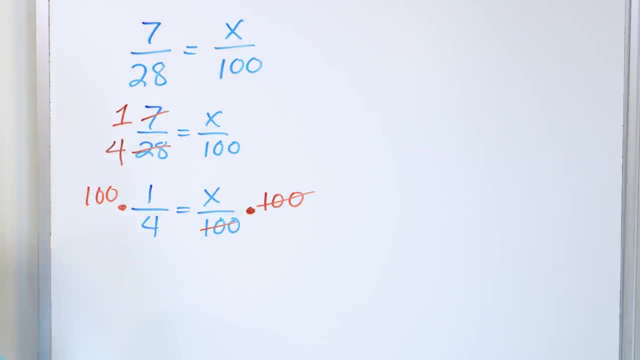 that the 100 will cancel with the 100 over on that side. So on the right you will have an x And on the left 100 times 1 in the numerator will be 100. And this will be a 4 times, Don't forget. 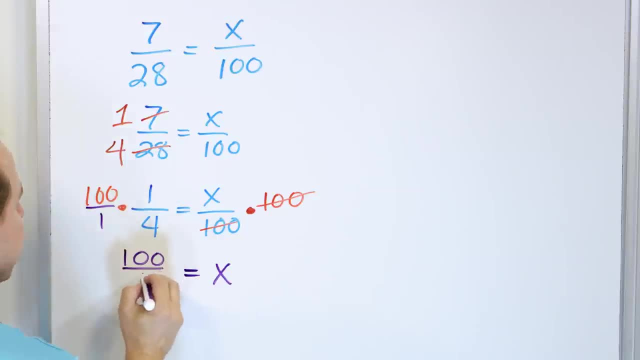 this is like an invisible over 1 here. So 4 times 1 is 4. And so x will be what's 100 divided by 4? 25.. x will be 25. And that means the answer is 25%, because x, this number here, is 25.. And 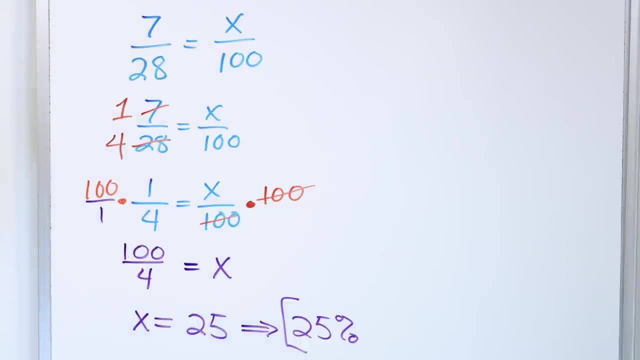 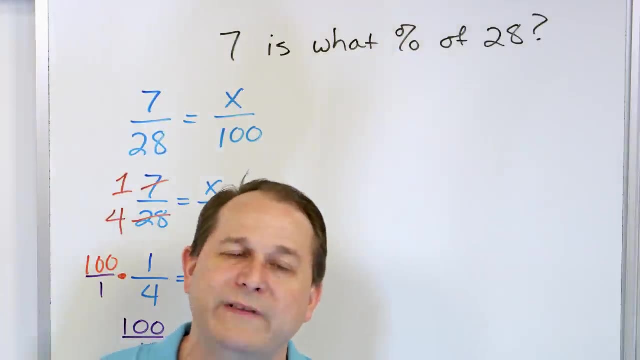 25 out of 100 is 25%. So what it means is: if you took 25% of this, then the answer is going to be 7.. And it makes sense because you know that 7 times 4 is 28.. So that means that to make 28,. 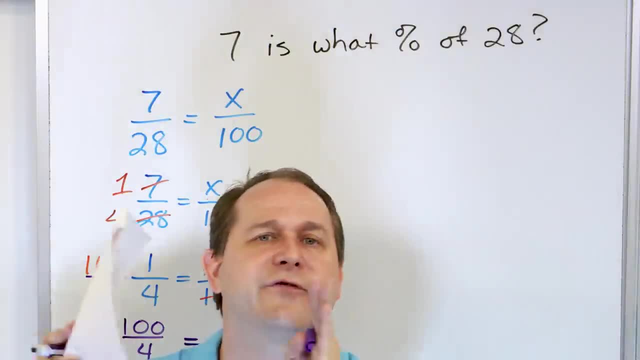 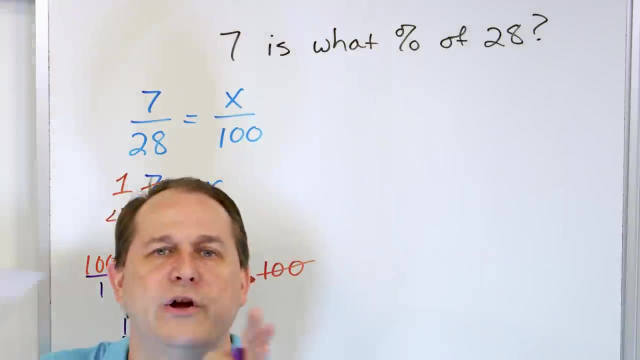 you could do 7 plus 7 plus 7 plus 7.. There's four groups of 7, because 7 times 4 is 28.. So 25% of that would be to take one group out, which would be 7.. So if we took this and divided, 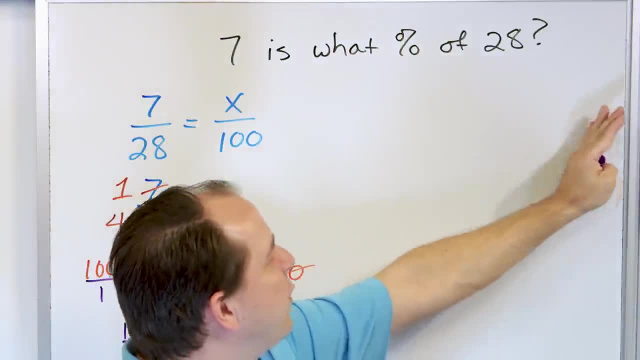 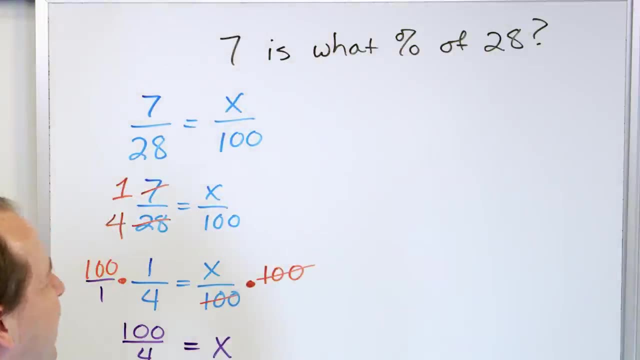 it into four equal groups: 25%, 25%, 25%, 25%. one of those groups will be 7, because 7 times 4 is 28.. So 7 is 25% of 20.. In other words, it's a quarter of that right. Half of this would be. 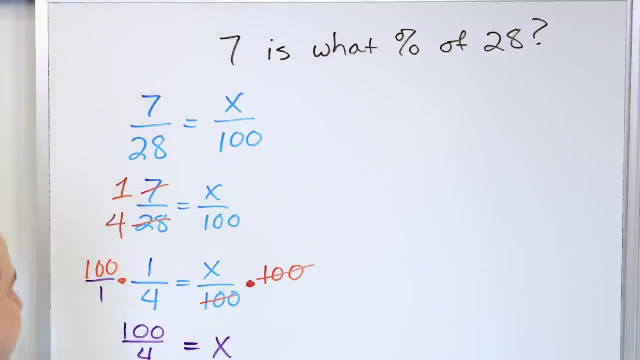 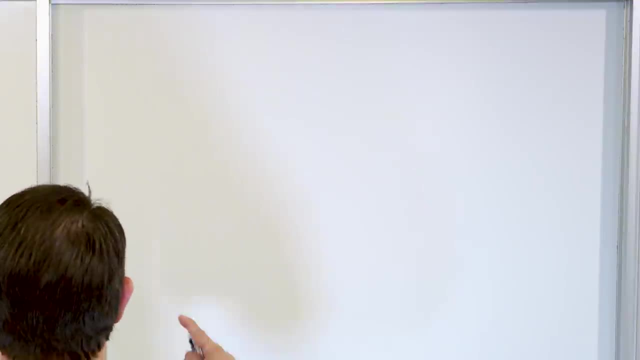 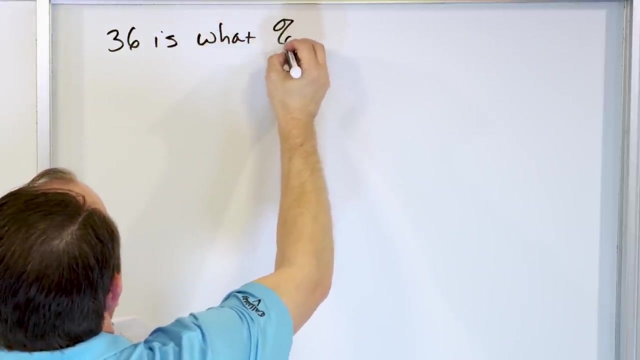 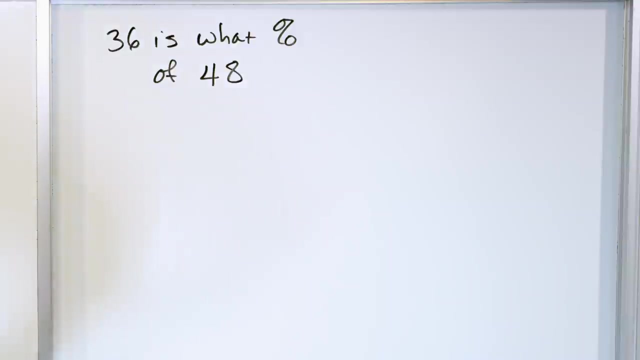 50%, which would be 14.. And so half again of that would be 7.. All right, let's take a look at problem 3.. Problem 3. 36 is what percent of 48?? 36 is what percent of 48?? We're comparing the. 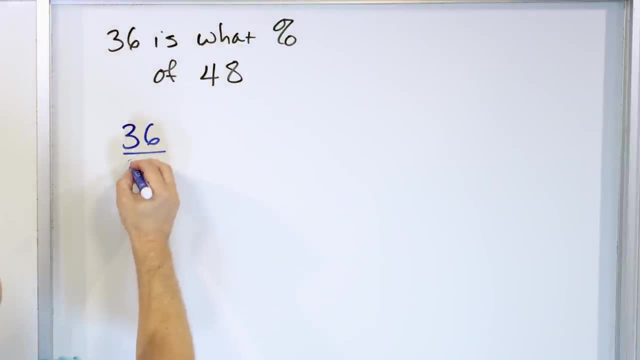 numbers 36 and 48. So 36,, as it compares to and relates to as a ratio with 48, is equal to- we're looking for- a percent, something over 100.. All of them will basically be the same form, like this: 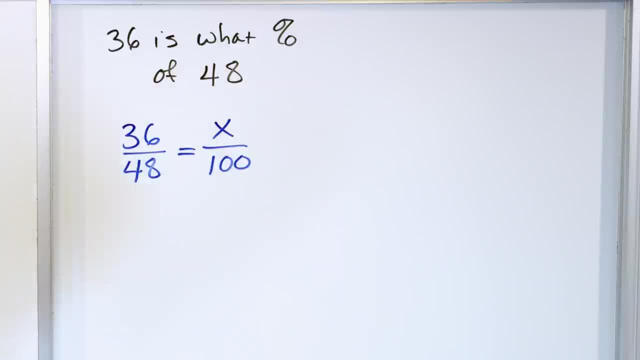 And I'm using x everywhere. but you can use a or b or d, It doesn't matter, I don't care what variable you use. Now let's rewrite what we have: 36,, 48, x and 100.. We could multiply by 100,. 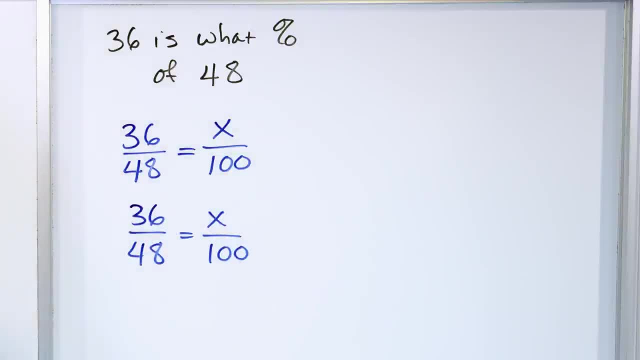 but notice how large the numbers are. We would have a lot of large numbers over there. So instead of doing that, let's just kind of pre-simplify: right: We know we can divide the top and bottom. We can divide by 2. That would help. 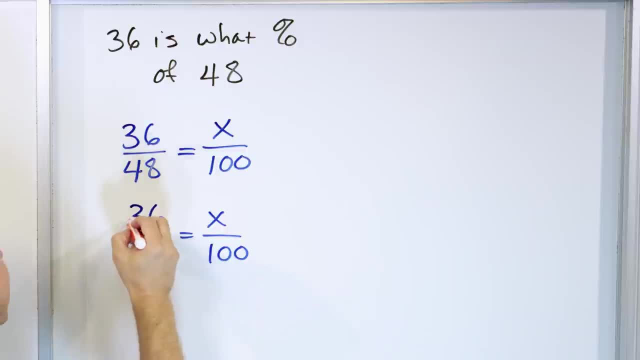 But if we think bigger, we can divide by 12, because we could divide this by 12 and get a 3.. We could divide this by 12 and get a 4, because 3 times 12 is 36, and 4 times 12 is 48.. 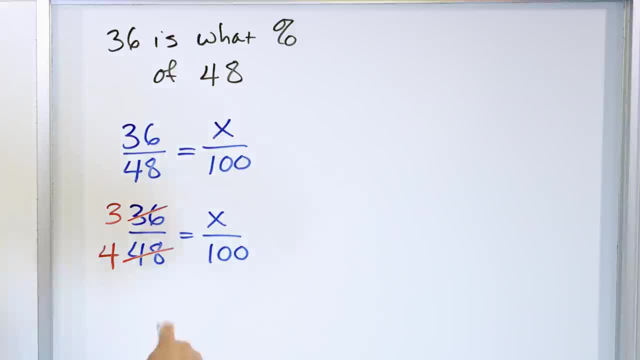 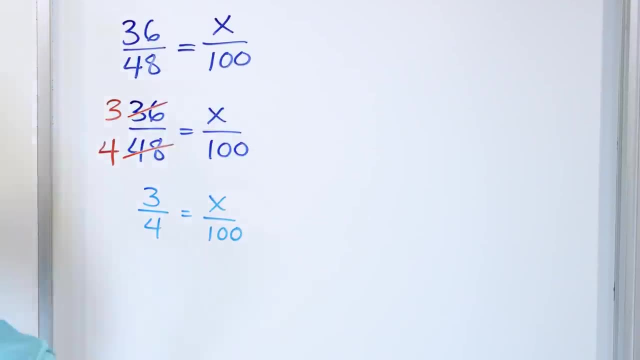 And now the problem is like much simpler to deal with, because over here on the left I just have 3 out of 4, and then x out of 100. So you don't have to do that step, but it does make it a lot easier. Here we're dividing by 100, so we'll do the opposite. 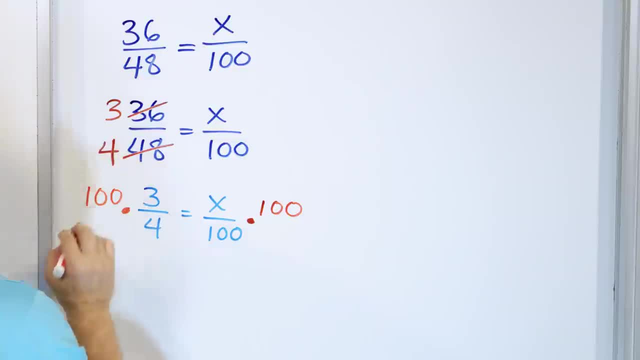 Multiply by 100, and we'll do it to both sides, obviously, to keep it balanced. And this 100 is like 100 over 1. It'll cancel because it's on the top. It'll cancel with this guy. And then what do we get On the right-hand side? just x by itself. That's what. 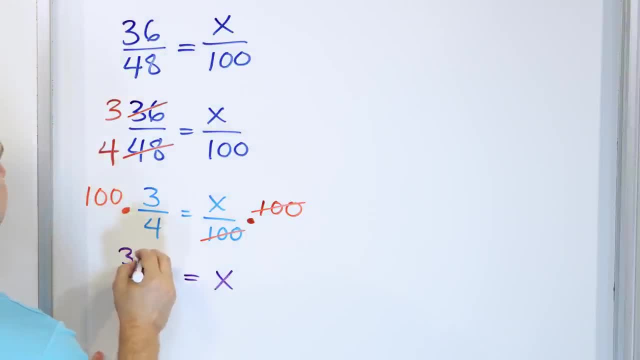 we want Here on the top 100 times 3 is 300. And then 4 times the invisible one here is a 4.. So we have 300 divided by 4, all right. Maybe you're not sure what the answer to that is. 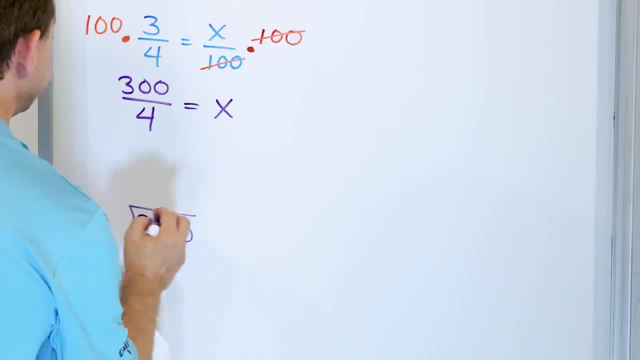 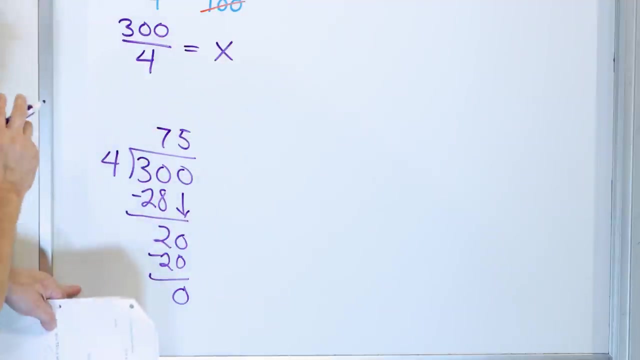 so just come down here and say: what is 300 divided by 4?? So 4 times what 7 is 28.. And then the difference there is 2.. Drag down another 0. And then 4 times 5 is 20.. And then now the remainder is 0. So the answer came out to 75. 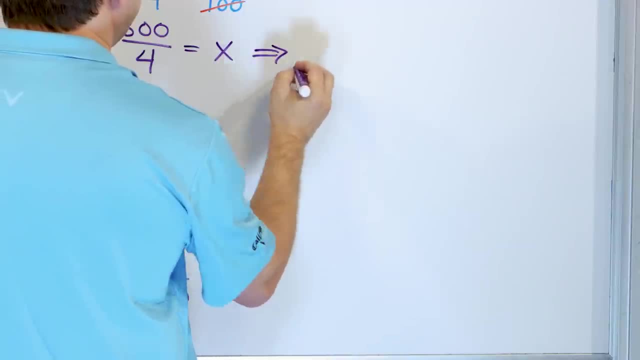 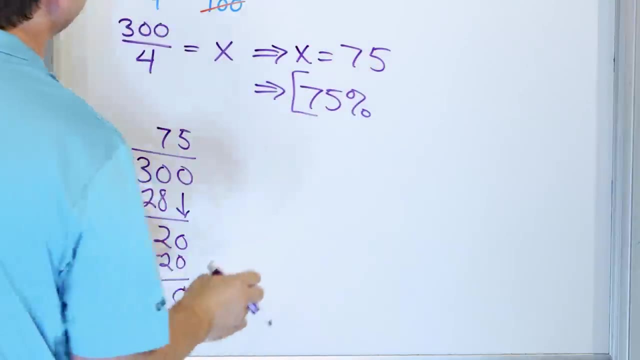 So we found out that x is equal to 75, which means that the answer in a percentage is 75%, because it was x over 100.. So what we figured out is 36 is actually 75% of the number 48.. 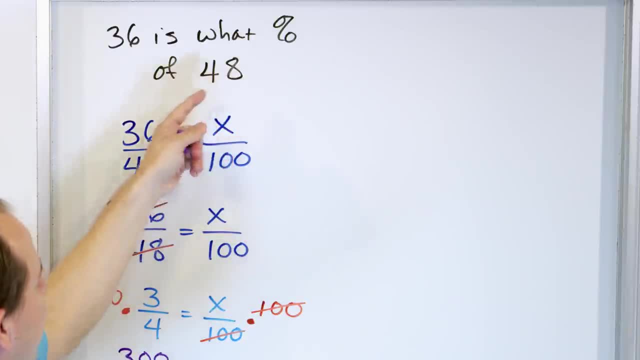 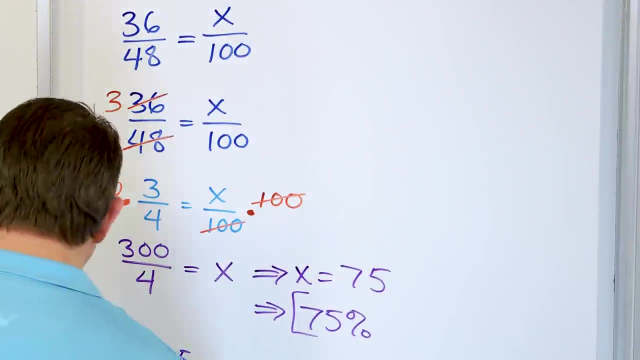 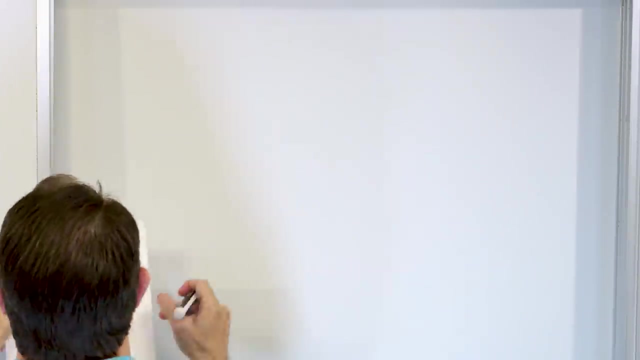 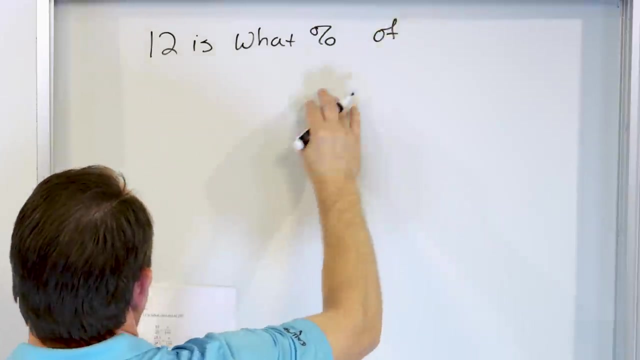 It makes sense, because half of this would be 50%. We're calculating way more than half. 36 is more than halfway there, So that does make sense for the answer. All right, let's calculate the next one here. Let's take a look: 12 is what percent of 20?? 12 is what percent of 20?? 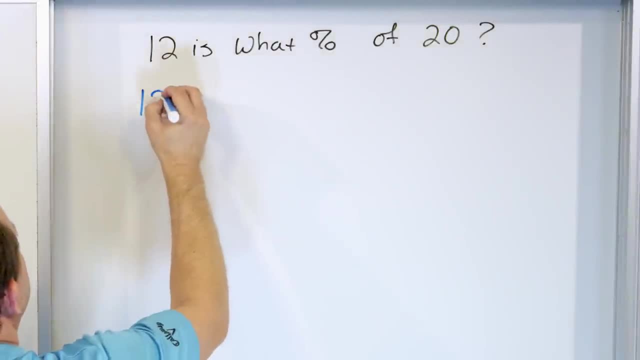 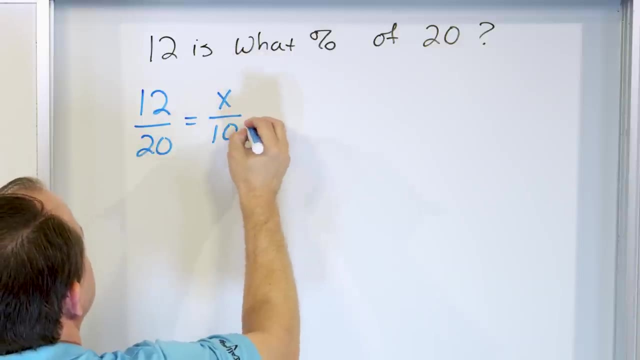 So when we translate basically, what we're saying is the number 12, as compared to the ratio of 20, is equal to x over 100. So let's rewrite 12, 20, x and 100.. Now we can simplify, We can pre-simplify. 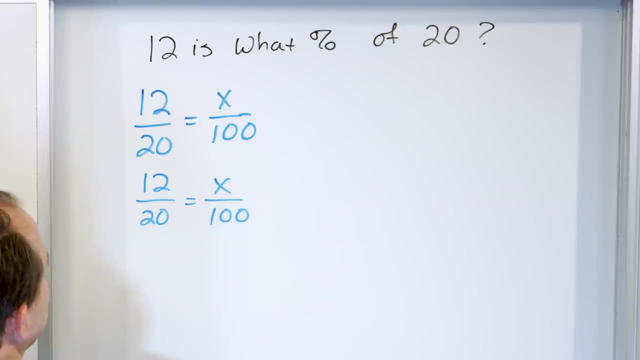 We know we can divide these guys by 2.. We also know we can divide by- let's see 4.. We can divide by 4, right? Because 12 divided by 4 is 3. And 20 divided by 4 is 5.. So we have a 3 and a 5 right. there, And let's rewrite the problem: 12 divided by 4 is 3. And 20 divided by 4 is 5.. So we have a 3 and a 5 right there, And let's rewrite the problem: 12 divided by 4 is 3. And 20 divided by 4 is 5.. So we have a 3 and a 5 right there, And let's rewrite the problem. 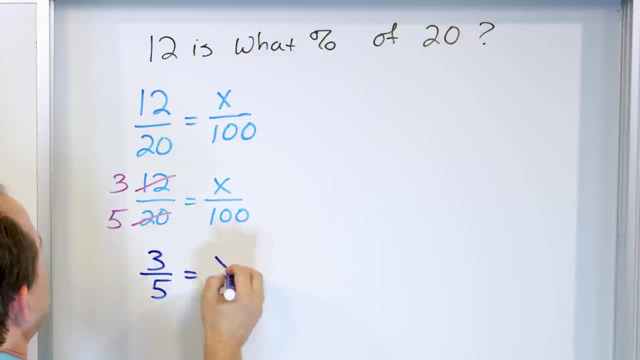 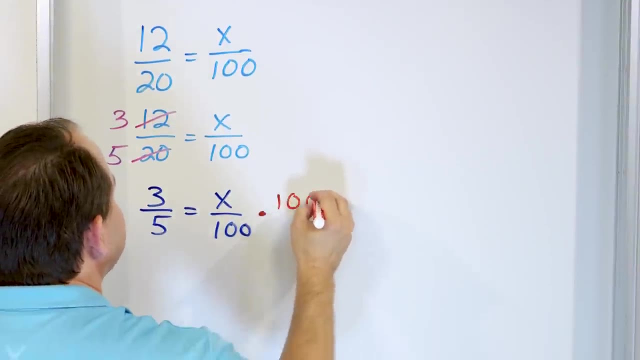 On the left, we're just going to have 3 fifths. On the right, x over 100. And just like every single one of these problems, we can multiply by 100 to get this by itself, and multiply this by 100. 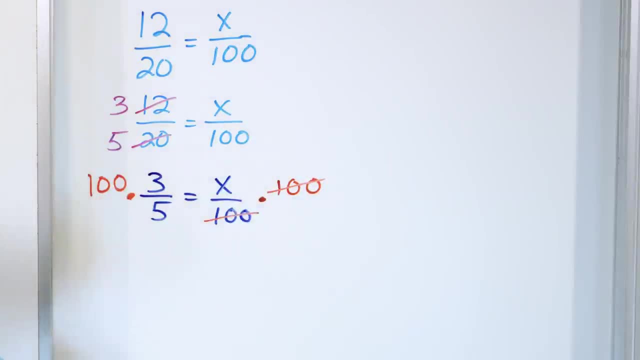 like this. So this 100 cancels. with this one, They divide away And on the right-hand side all you're going to have is just x by itself. Here on the top, 100 times 3 will be 300. 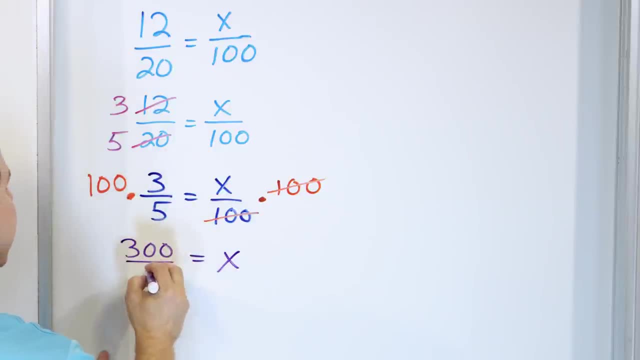 And the 5 times the invisible 1, because this is a fraction over 1, is just 5.. Right, And so if 30 divided by 5 is 6, then 300 divided by 5 has to be 60.. You can do the long. 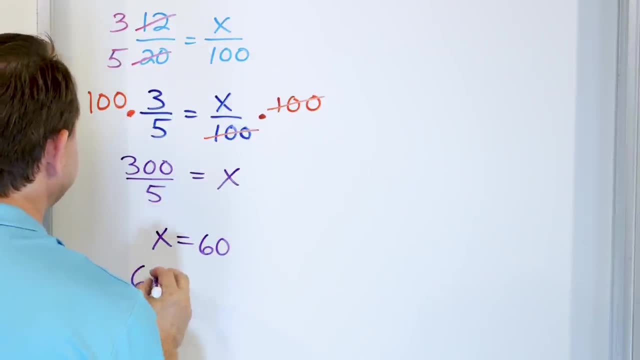 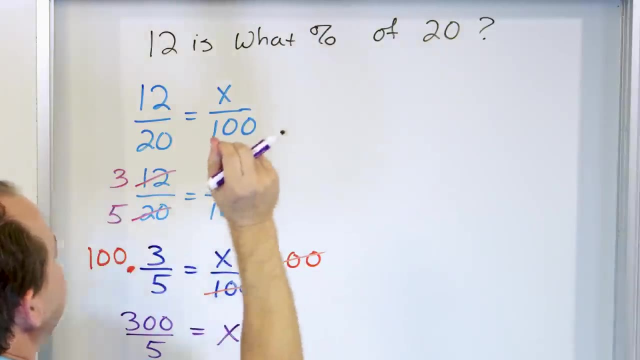 division to prove that to yourself. But since you have 60, the answer is 60%, The answer is 60%. So what we figured out is 12 is 60% of 20.. Does it make sense? Well, 20, exactly half of it. 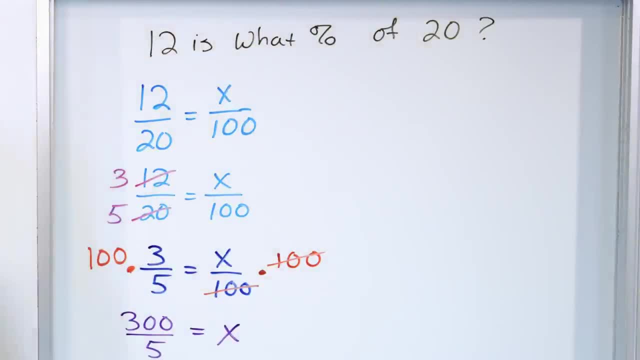 50% would be 10.. But we're not. We said it was 60%, So it has to be more than 10.. So, and 12 is more than 10.. So it makes sense that 12 would be more than 50% of this. 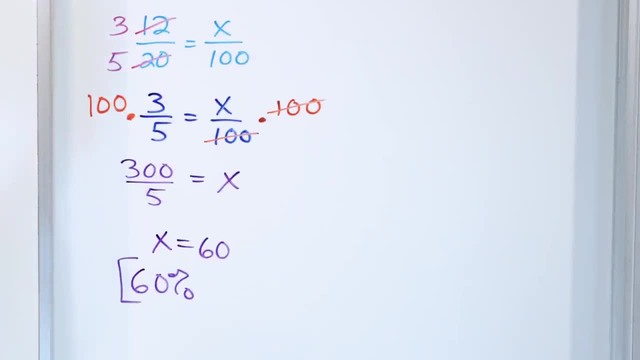 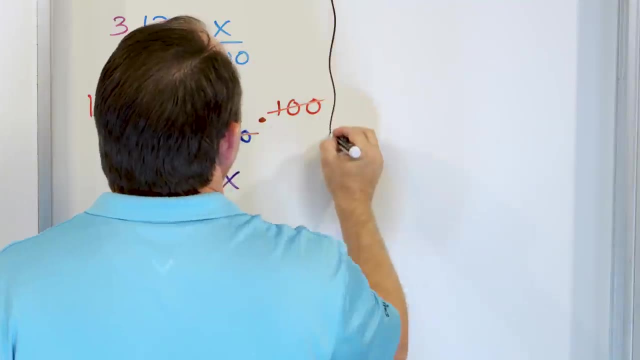 because 50% would be 10. And, of course, 12 is bigger than 10.. All right, I think we're only going to do a couple more. Let's squeeze one in here and then one on the other board, And 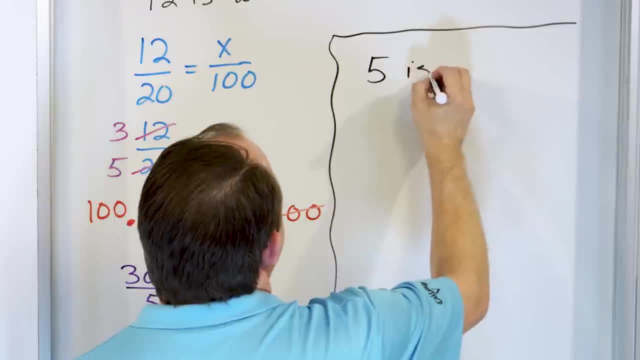 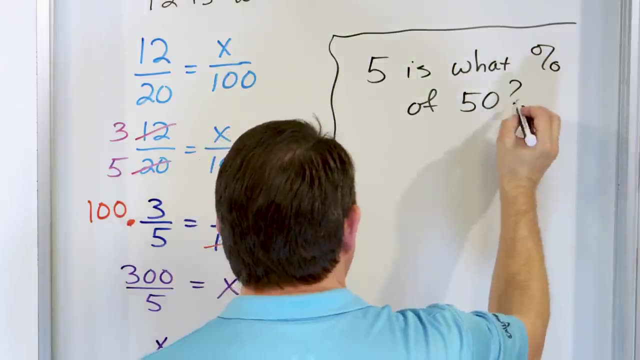 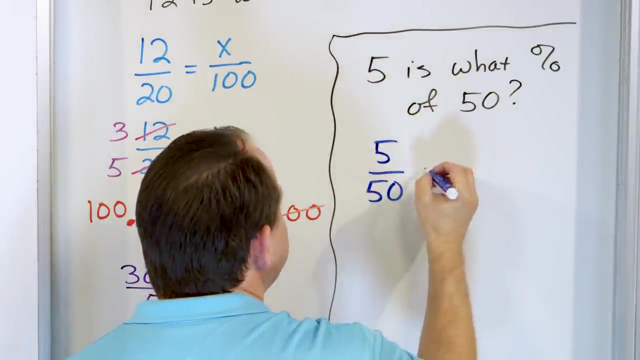 I think we'll just call it a day. 5 is what percent of 50? Right? So what we're asking is: what is the ratio of 50 to 50?? And we're comparing 5 and 50.. We'll say 5, as it compares to the. 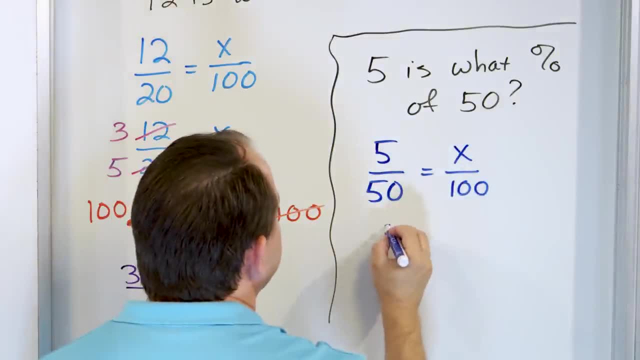 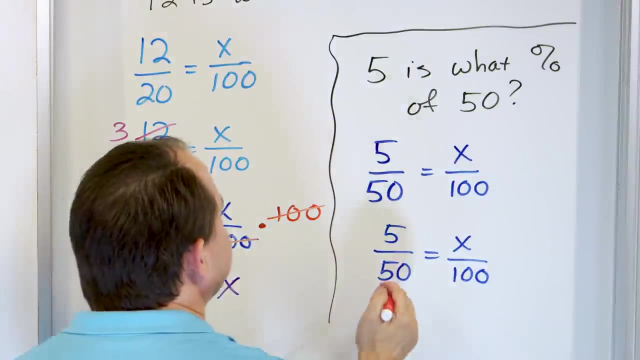 ratio with 50, is some number over 100.. We're trying to find the percentage, So let's rewrite 5, 50, x 100.. All right, So we can pre-simplify here: Divide by 5.. 5 divided by 5 is 1. 50. 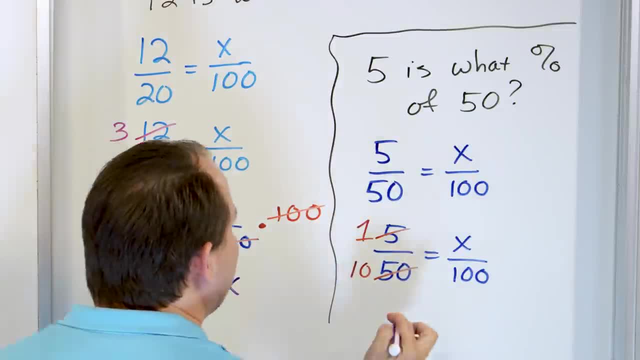 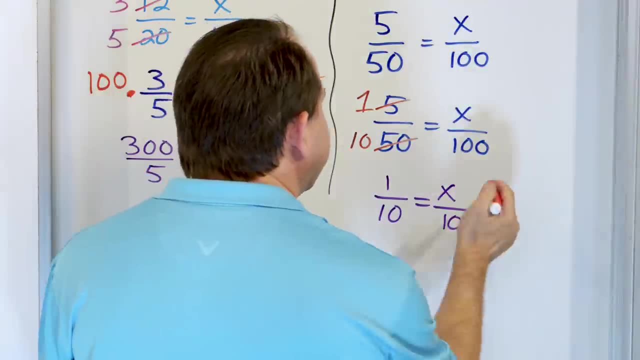 divided by 5, 10.. And so when we rewrite, we're going to have 1 tenth on the left, x over 100, on the right, And I can get x by itself. I'm dividing by 100. So I'll do the opposite. 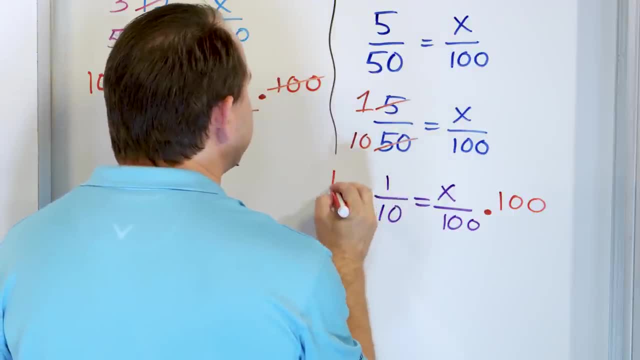 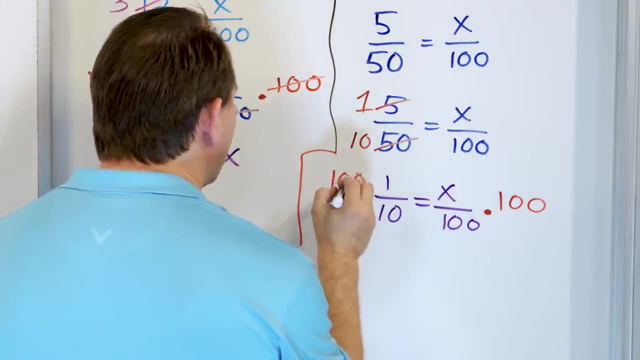 Multiply by 100. And I have to do the same thing to both sides. Multiply by 100 to make it equivalent. Now, on the left-hand side, I have 100 times 1, which is 100. And then 10 times the. 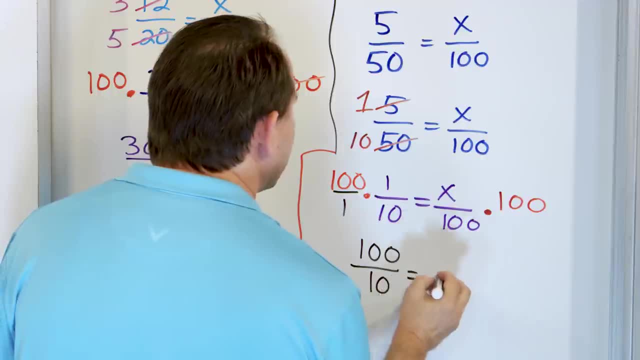 invisible 1, because this is like over 1, is a 10.. And then, on the right, these cancel, which just leaves me with x, And so x is going to be equal to divide 100 by 10, is 10.. 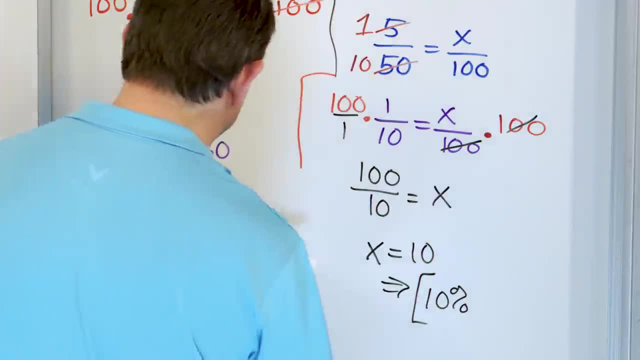 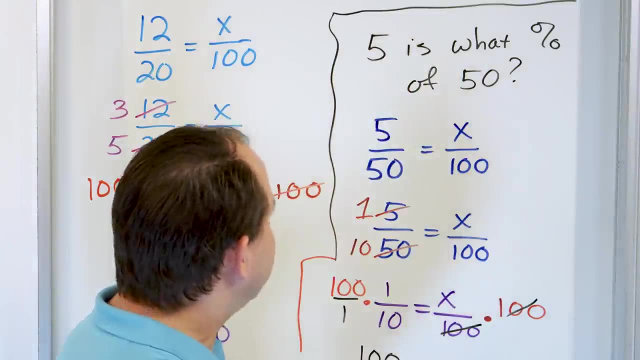 Which means it's 10% because x over 100, right, It's 10%. So what we figured out is that when we're comparing 5 to 50, it's exactly 10% of 50, right, 10% of 50.. And that's the final answer. 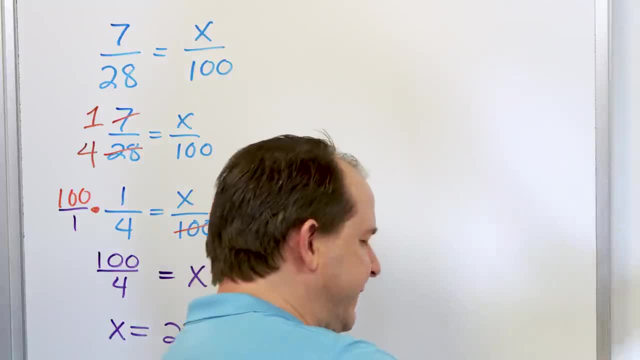 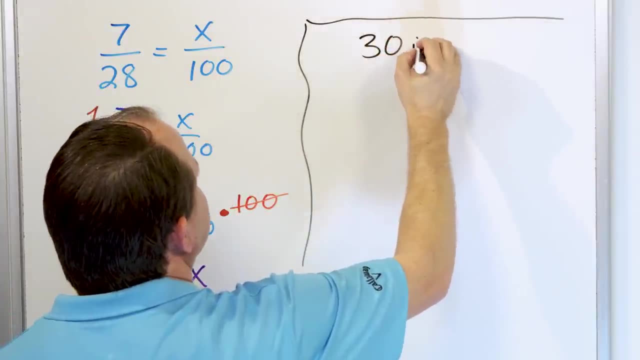 All right, We have one more on this one And I think we're going to call it a day. Let's just go ahead and solve it. I guess we'll just solve it like over here. Let's say, 30 is what percent of? 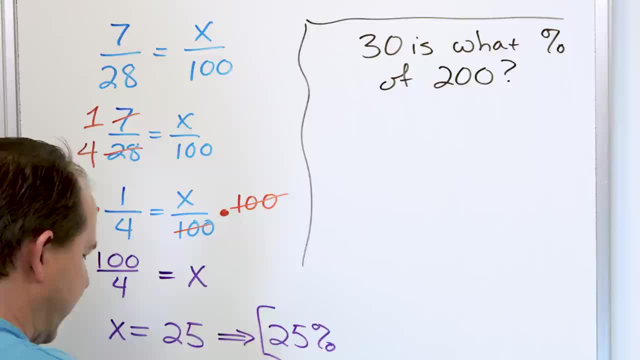 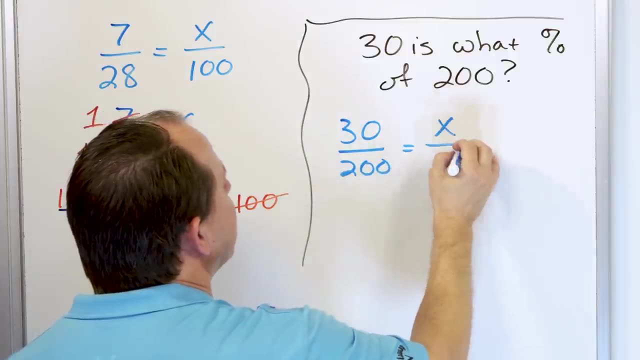 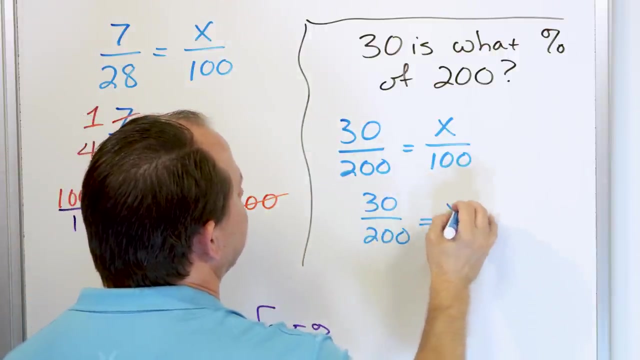 200? 30 is what percent of 200?? What we're saying is that 30, as it compares to 200, is equal to some unknown number as it compares to 100, right? So let's rewrite 30 over 200 x 100. 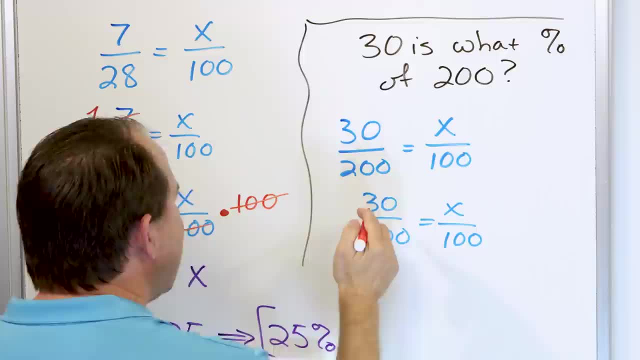 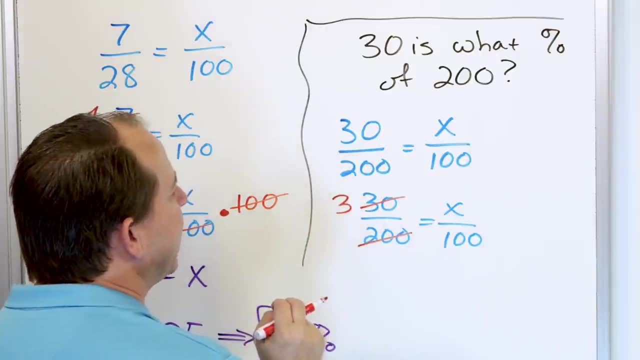 I'm rewriting so I don't flash through all of my original stuff. So I can simplify these right, Because I can divide top and bottom by 10.. 30 divided by 10 is 3. And 200 divided by 10 is. 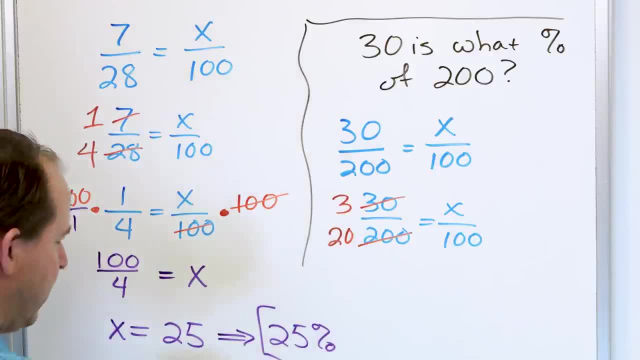 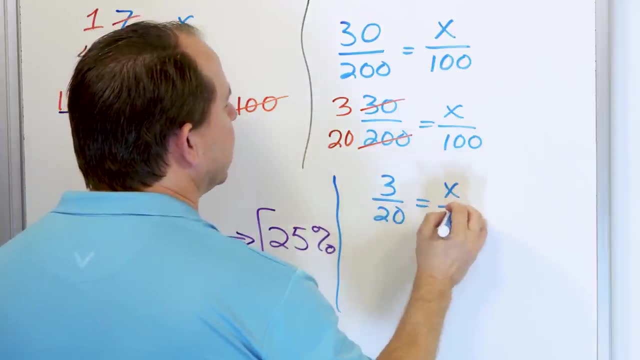 20.. So I'm dividing top and bottom by 10.. So let's rewrite the problem And over here we're only going to have 3 out of 20, or 3 over 20 x 100.. So I multiply on the right-hand side by 100. 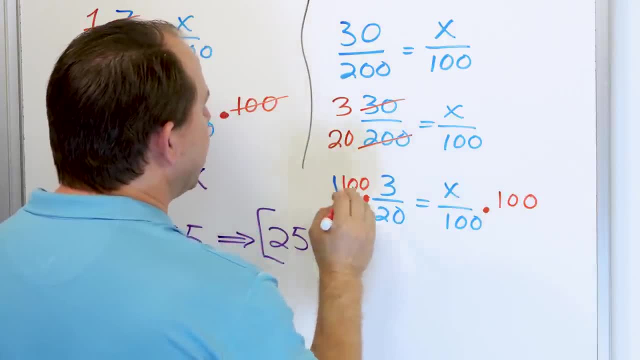 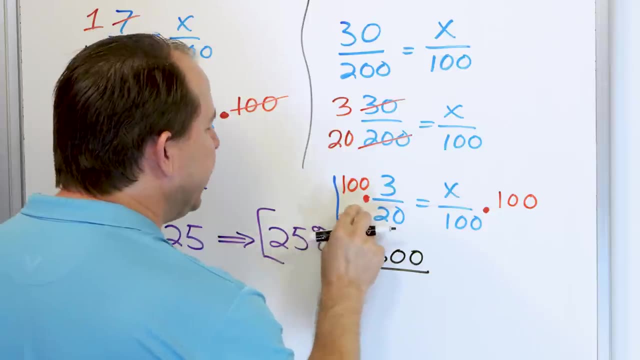 to kill it down here, And I have to do the same thing over here. Multiply by 100. So on the left-hand side, 100 times 3 is 300. And then 20 times the 1- here invisible is right down here. And then these: 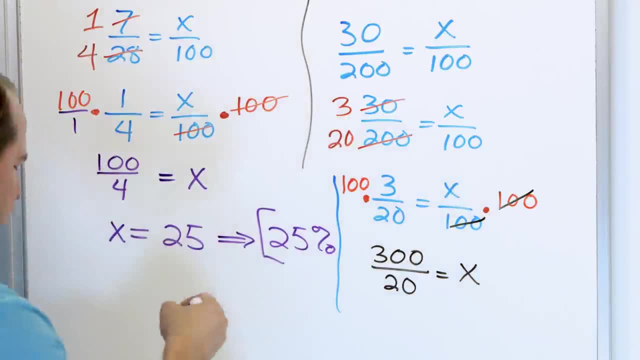 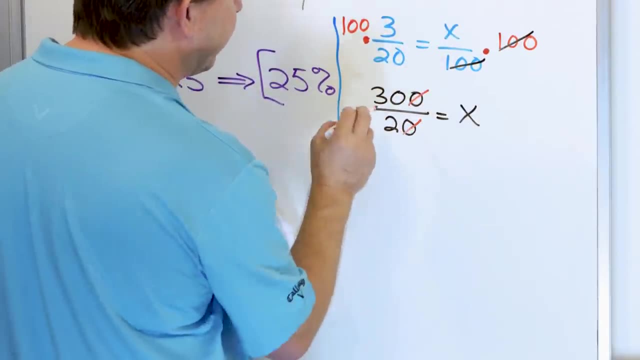 100s cancel And you have x on the right. right Now we have to take 300 and divide by 20.. We can cancel the trailing 0. So it's really 30 divided by 2. And we can say x is equal to 15.. 30 divided.